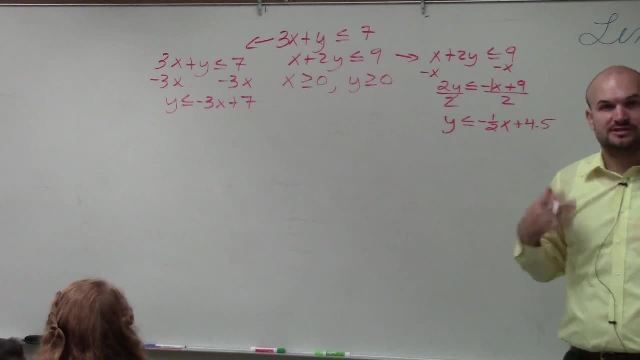 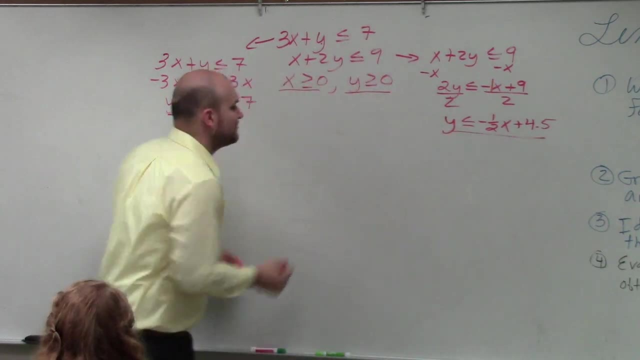 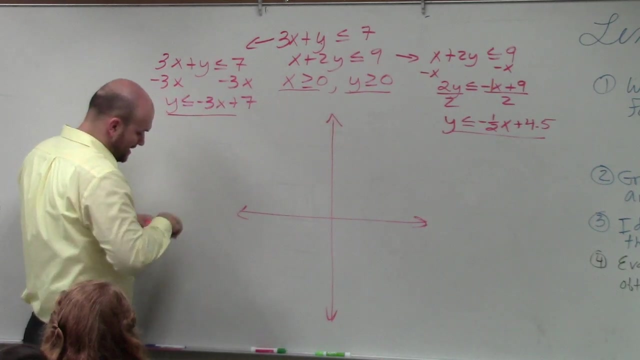 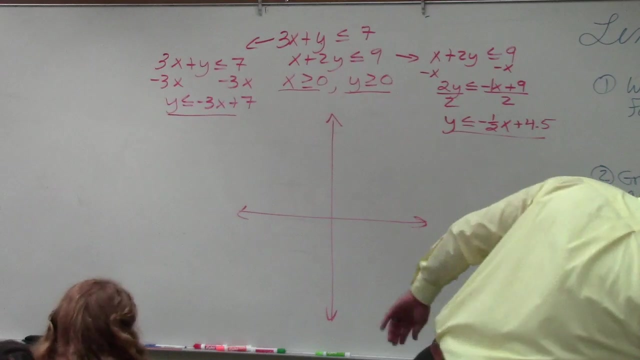 we've covered. It's just solving for y. I know if you have trouble with this, you just need to practice. All right, So now we have three, four equations we're going to graph. So first equation: It has a y intercept at 7 and a slope of negative 3.. I want a black. It has a slope of negative 3. 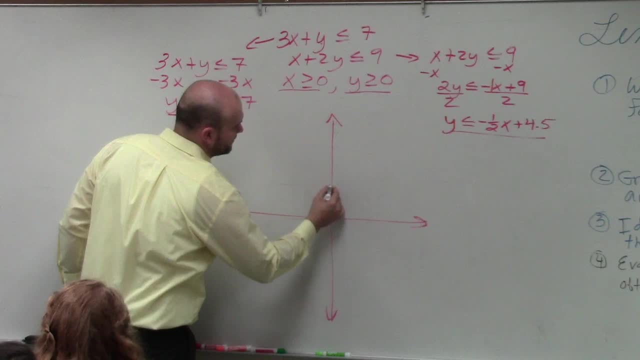 over 1. So I go up to 7.. 1,, 2,, 3,, 4,, 5,, 6,, 7.. And I go 1,, 2,, 3.. I go down 3 to the right, 1. Down. 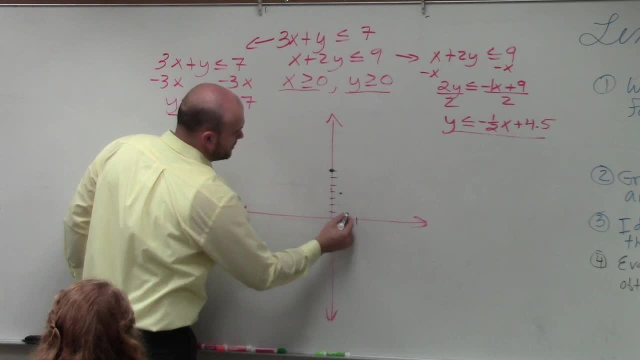 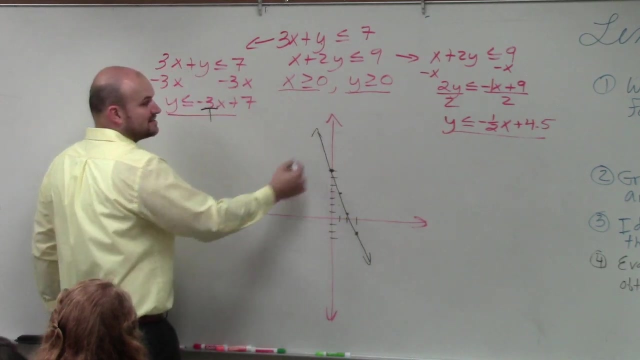 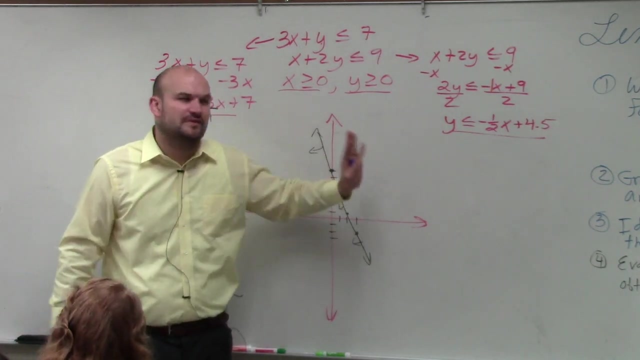 3 to the right, 1.. Down 3 to the right, 1.. Now this is going to make a four. I move up 2, so it's going to give me one plus 1 cancels that. So I'm gonna use two, three, four, 5,, 6,. 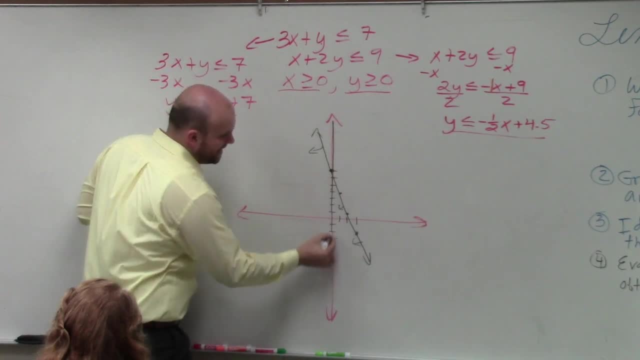 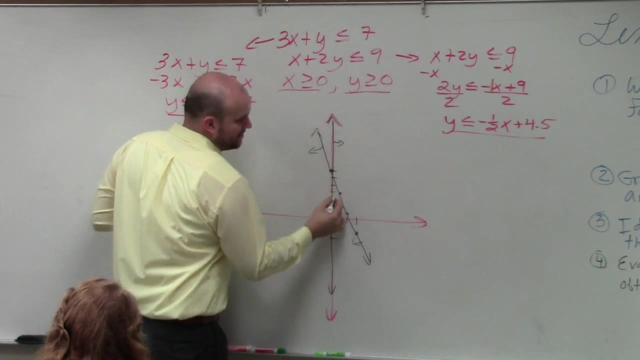 1, 2,, 3, 4,, 5,, 6, 7.. Now, I'm a linear, So it's going to look something like that. It's less than or equal to. So I know that since it's less than or equal to, I'm going to shade below the line Right. 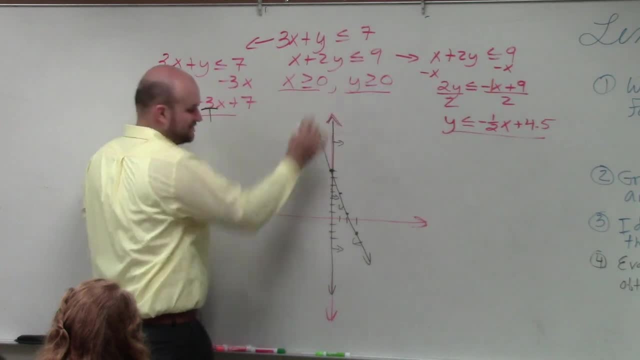 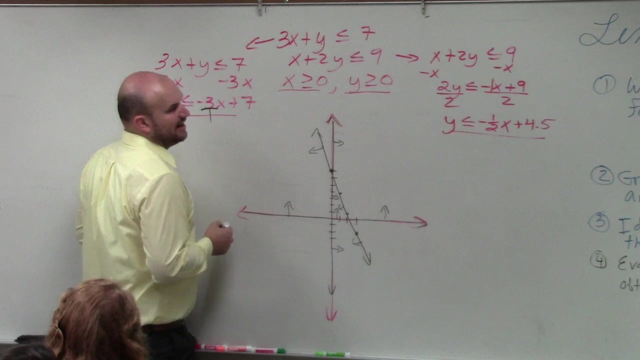 shade to the right, y is greater than or equal to 0. That's a horizontal line And all values of y that are greater than 0 are going to be above, And the last one is 4.5 plus negative 1 fx. 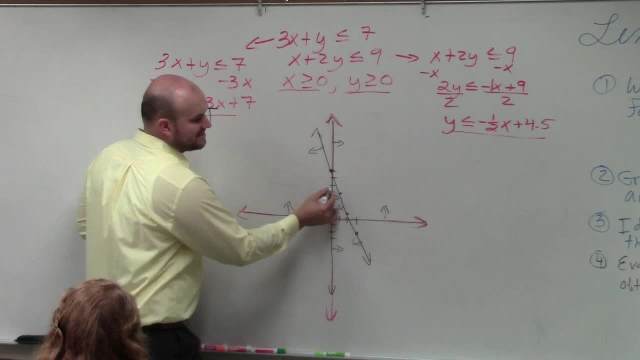 So I go up to 4.5.. 1,, 2, 3, 4.. 4.5 is in between. Then I go down: 1 to the right, 2. 1, 2.. You guys can see it looks like it intersects. 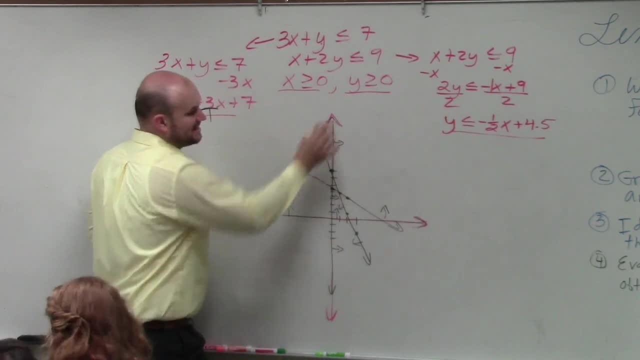 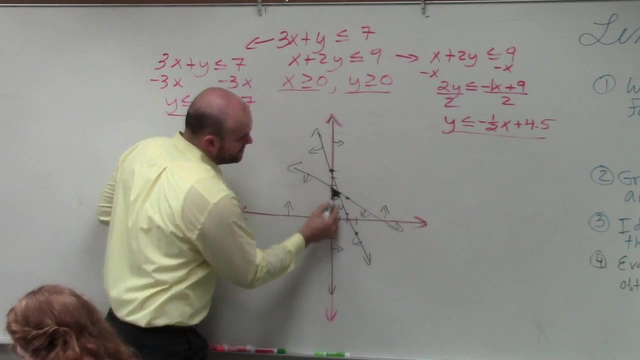 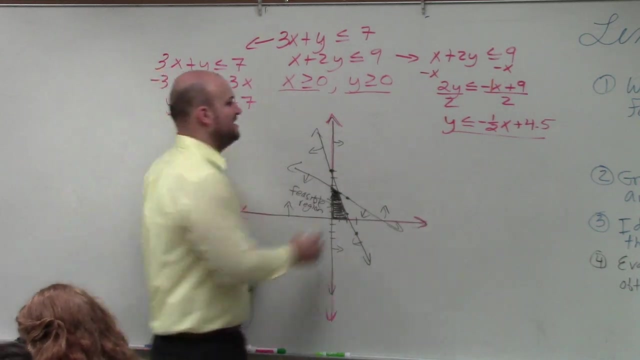 right at that point, Then that is less than so. it's going to shade below. So what you guys can do is determine that my feasible region is this little shape right here. So if you have a feasible region now, we need to identify the vertices. 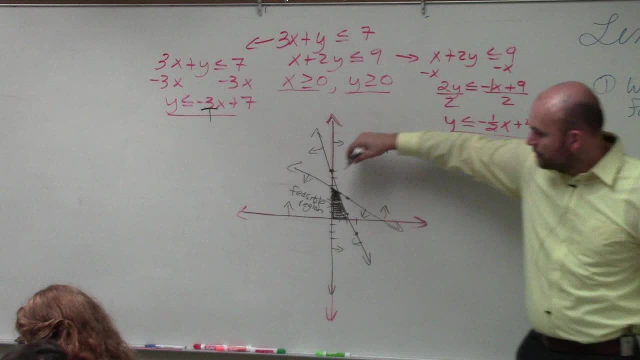 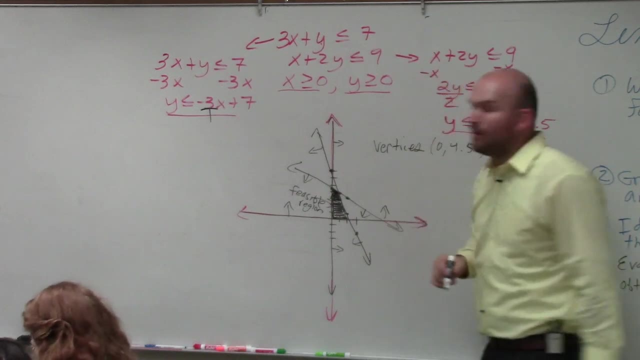 So the vertices are where each and every point of this line intersects. So you're going to go down the line and the first point you're going to see is where your inequalities intersect. So the first point that I have here is 0, 4.5. 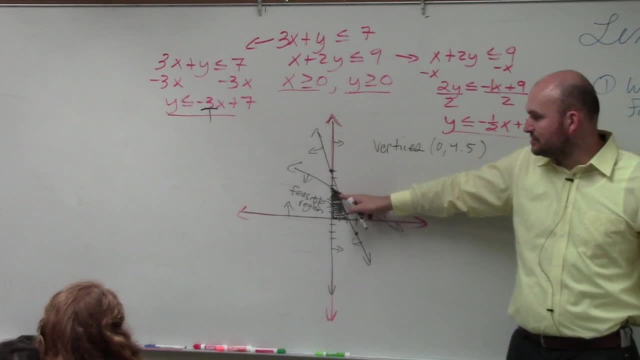 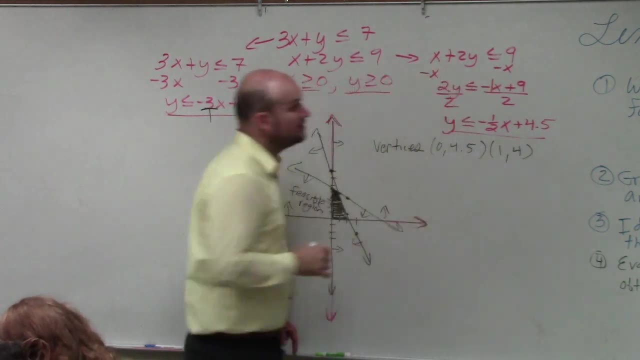 That was the y-intercept of that equation. right. It intersects at the y-intercept right there. The next point was the intersection of these two lines, which was positive: 1, 1,, 2,, 3,, 4.. 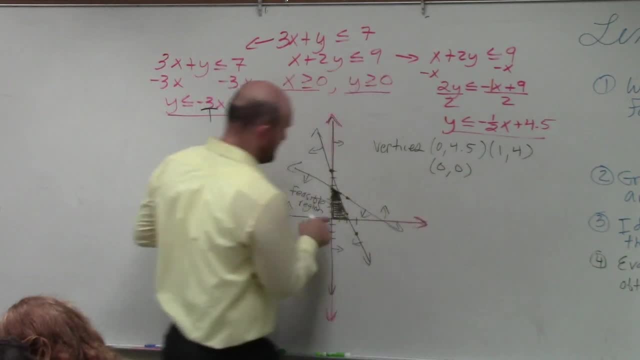 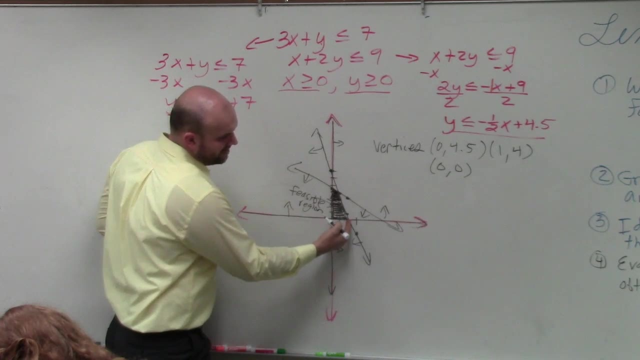 So I have 1, 4.. The next intersection is at 0, 0.. And then the last intersection is at 1, 2.. It's not 2,, it's not 3.. I'm going to say it's in between. 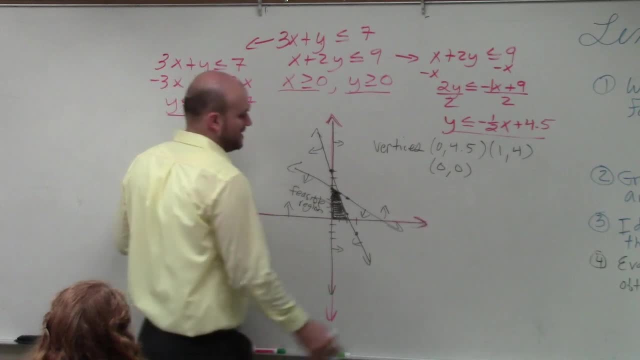 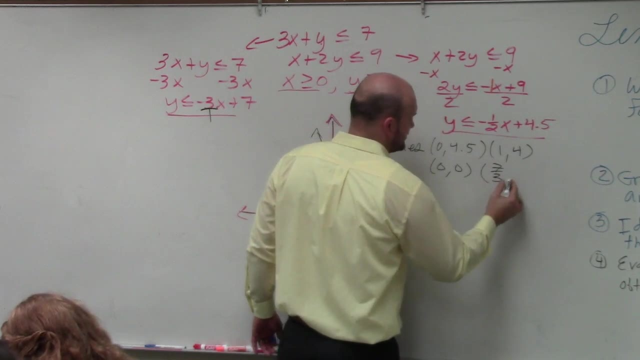 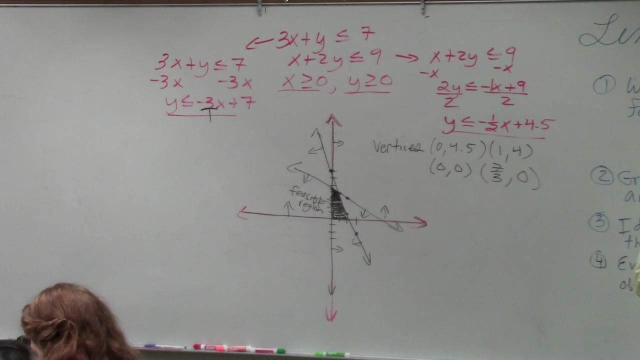 So it's not 1 third, So let's just say 2.3.. I think the answer in the book was 7 thirds 0.. OK, Now hold on. So the last problem. so does everybody see what I did? 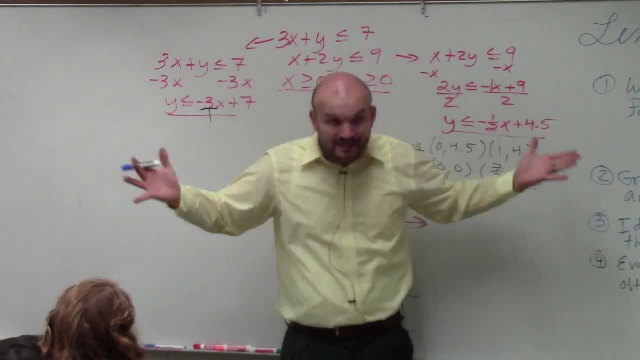 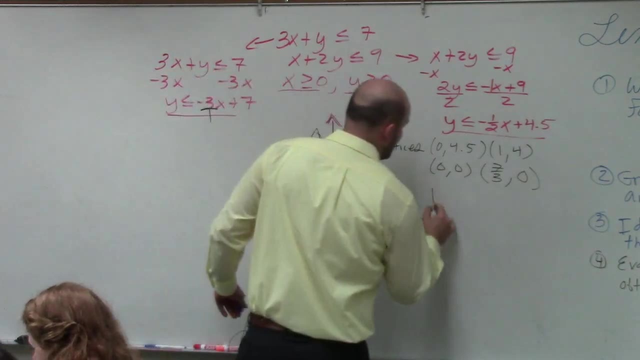 That's what I wanted you guys to do from step 3.. The last step, the only thing new that you guys are really learning, is: now we've got to evaluate for the objective function. And the objective function, they said, is they want you to evaluate for p, which 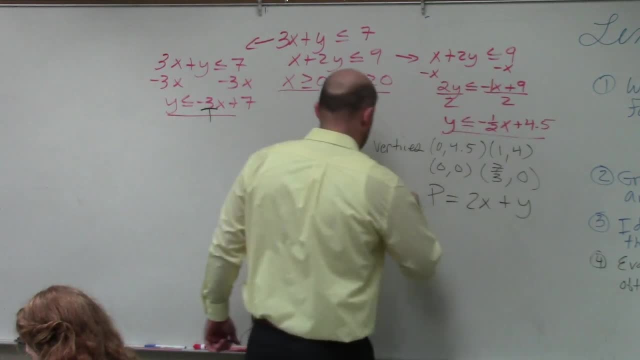 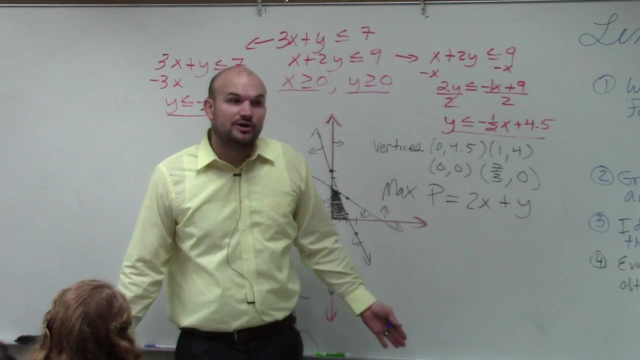 is: they want you to find the maximum of 2x plus y. They want you to find the max. So now do you guys see how I have four coordinate points? Yes, So what you're going to do? hold on, I still got time. 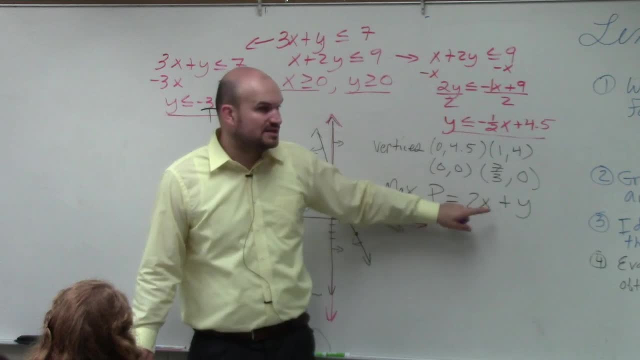 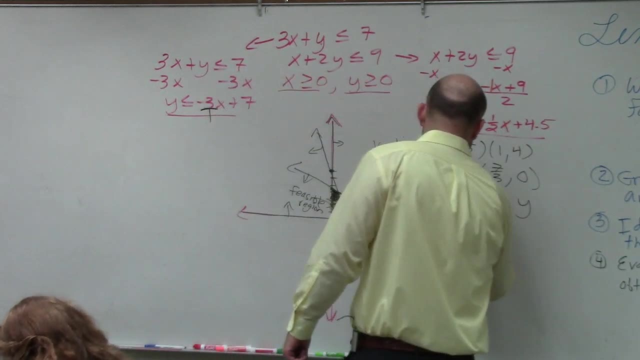 What you're simply going to do is plug in each and every one of these points for x and y and determine which one gives you the maximum p value. So let's do the first point. First point will be 2 times 0 plus 4.5.. 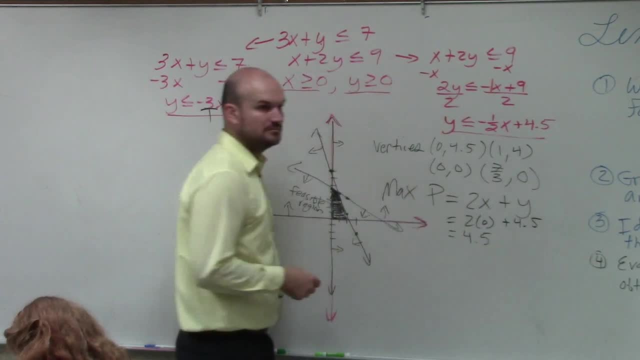 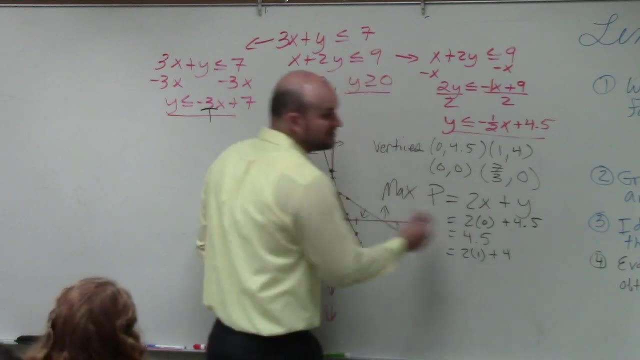 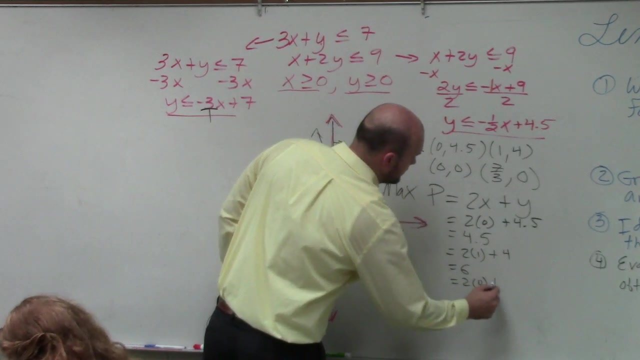 Well, that equals 4.5.. Next point is 2 times 1 plus 4.. 2 times 1 is 2 plus 4 is 6.. The next one is 2 times 0 plus 0.. Well, that's just going to give you 0.. 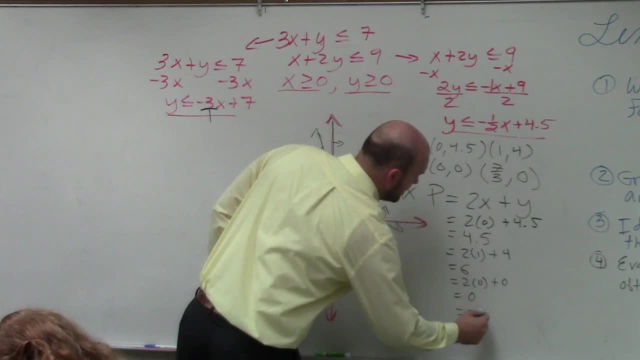 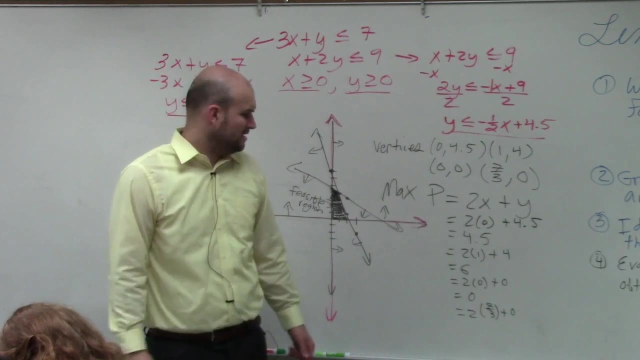 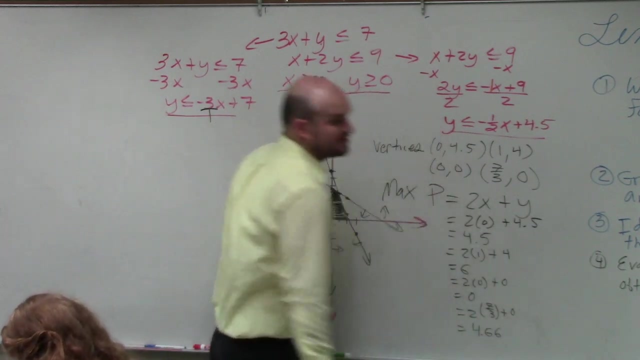 And the last one is going to be 2 times 7 thirds plus 0.. Well, 2 times 7 thirds is going to be 14 over 3, which would be 4 and 2 thirds, which is like 4.66 repeating. 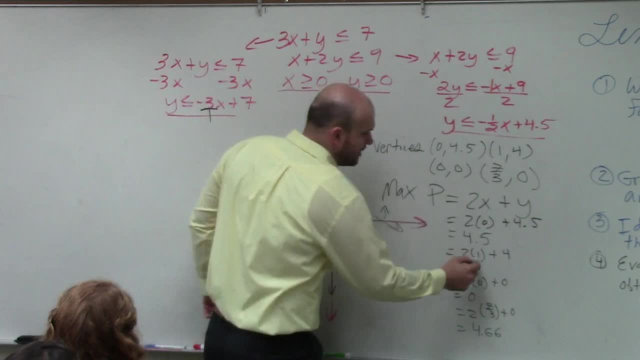 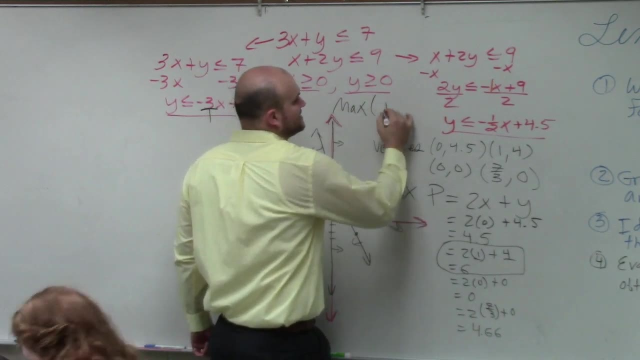 So what is going to be my largest value? The 1 comma 4,. right, That gives me my maximum value, p. So the max vertices is at 1 comma 4.5.. The max vertices is at 1 comma 4, where p is equal to 6..